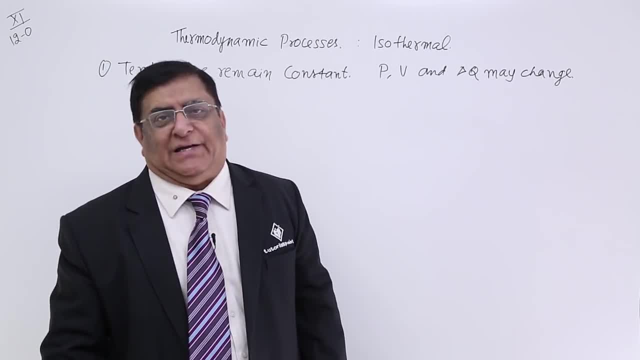 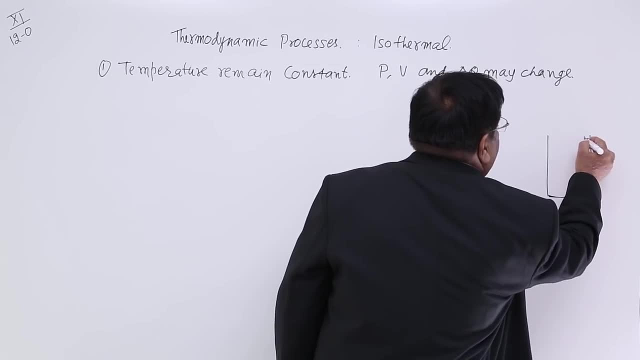 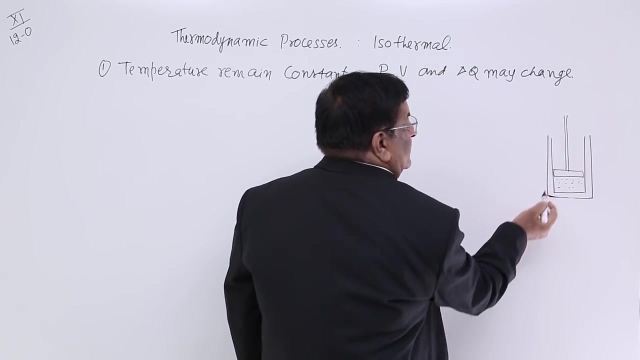 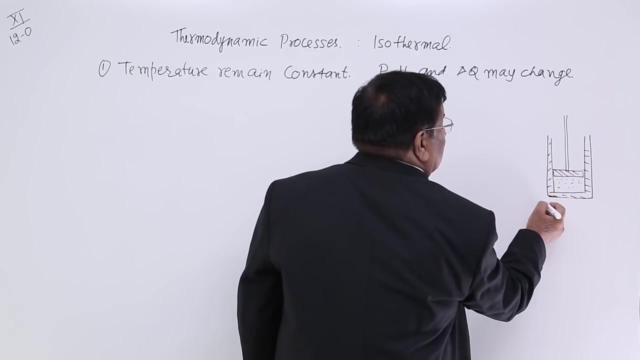 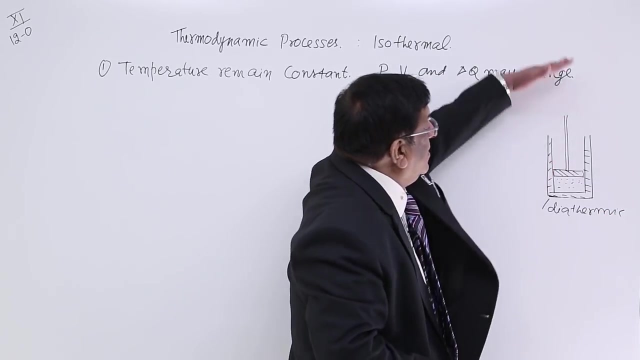 Then this process is isothermal process, How this process can take place. So here we have a piston and in this piston and cylinder system, here are the gases. This is piston. The piston can be moved up and down This wall. we take this wall as diathermic. Now, when we press it, what happens? 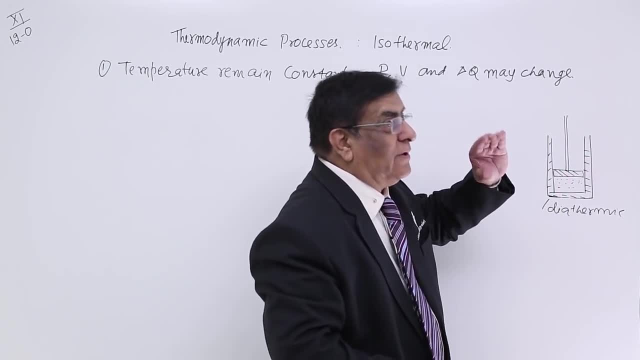 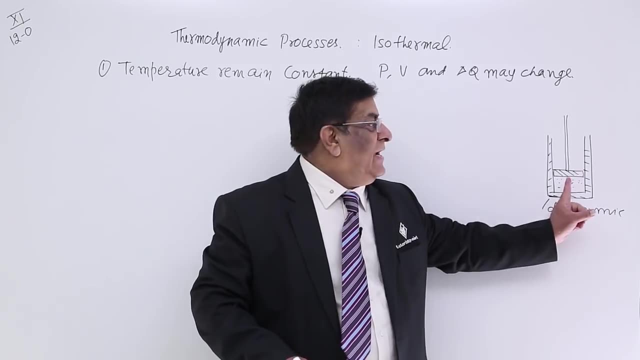 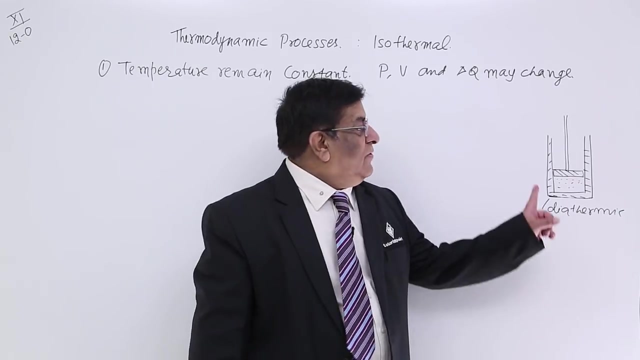 The pressure will become more. When the pressure is more, heat is generated here. with the change in pressure, with the compression, and that heat generated will rise the temperature. But what we do? We use this wall as diathermic wall as soon as the temperature rise. 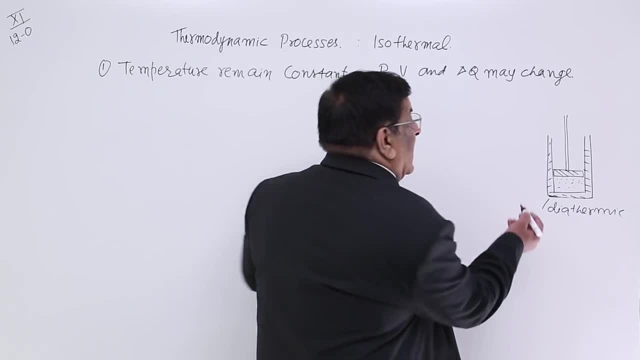 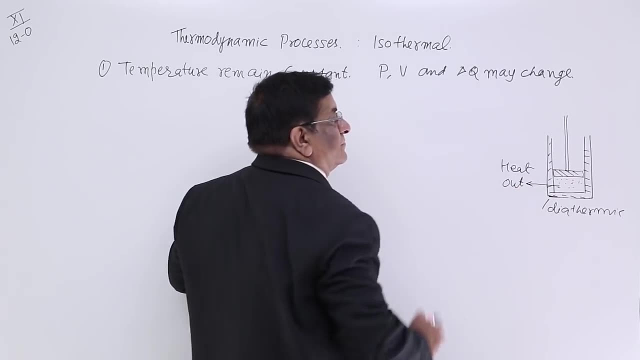 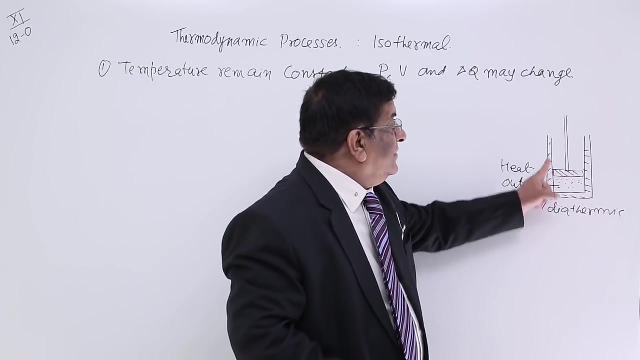 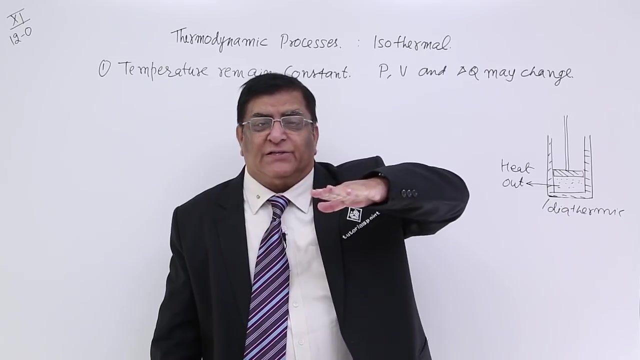 There is a change, There is a difference in the temperature and the heat comes out. Heat out What we have done Compressed, Press it So compressing, Compressing, using diathermic wall- the heat comes out. suppose we think that we press it so fast the heat does. 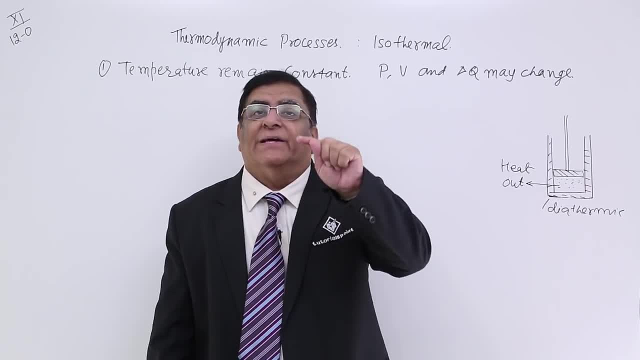 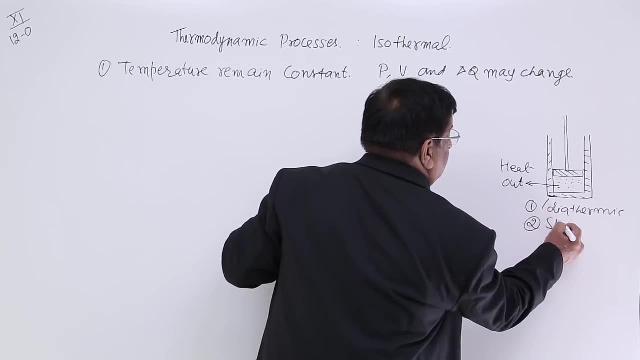 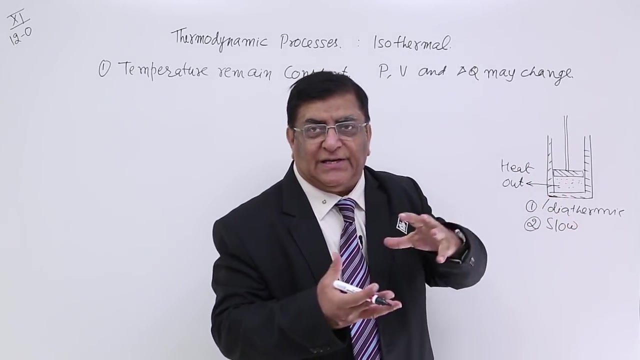 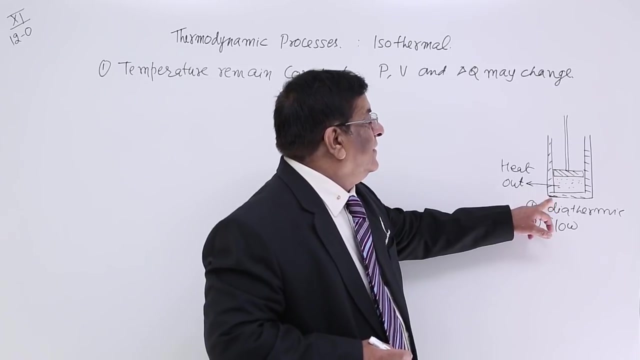 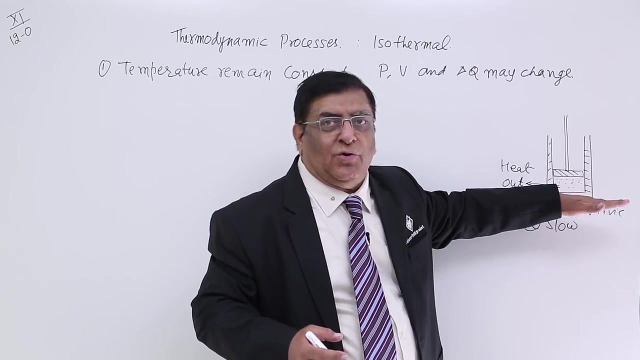 not come out, then we change our process. we make it slow, process slow. when we make it slow, then we press it slowly. certain heat is generated because of that temperature rise and that temperature leaks out because the wall is diathermic. so the temperature again comes back to the normal light atmosphere. again. press it a little more, again temperature try to rise. 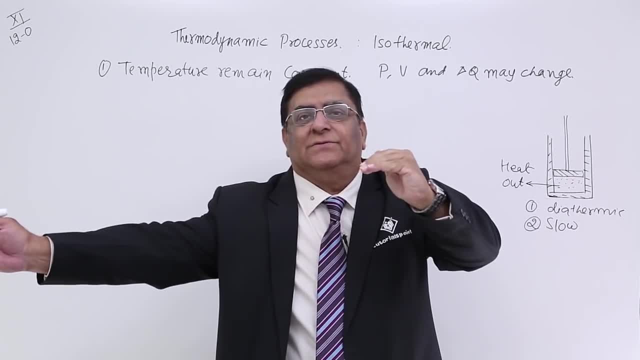 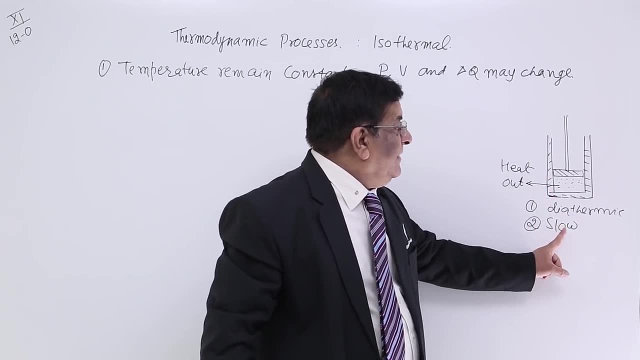 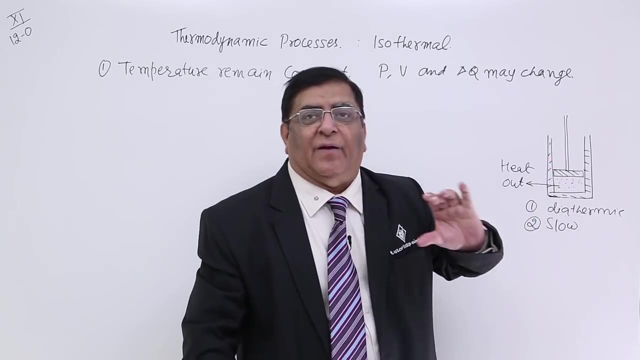 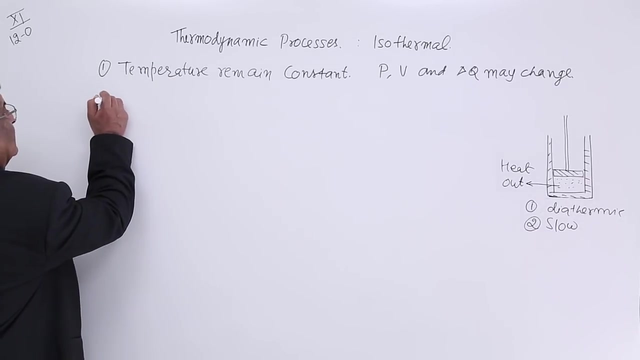 the moment it rise, the heat goes out and again the temperature become equal to the surrounding. so in this way, if we keep it slow, if we use the wall diathermic, then this process, temperature, can be kept constant, and this process will be known as isothermal process. so I write here slow process. 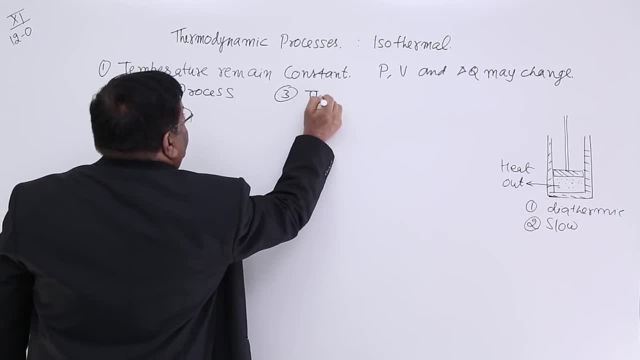 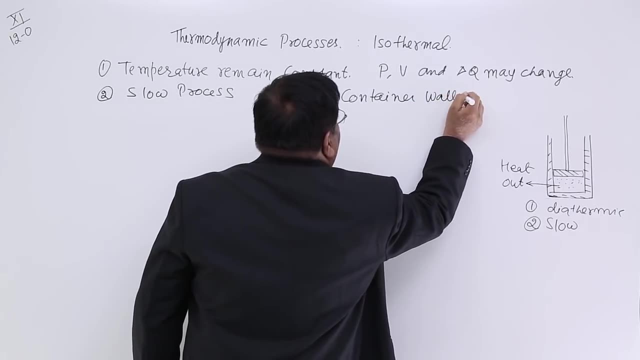 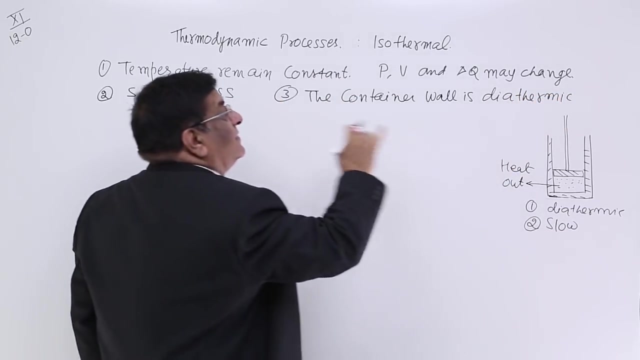 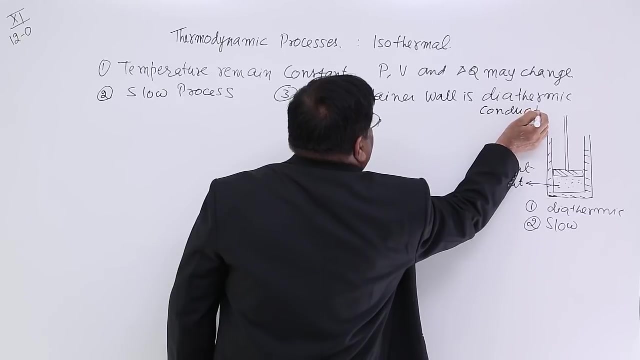 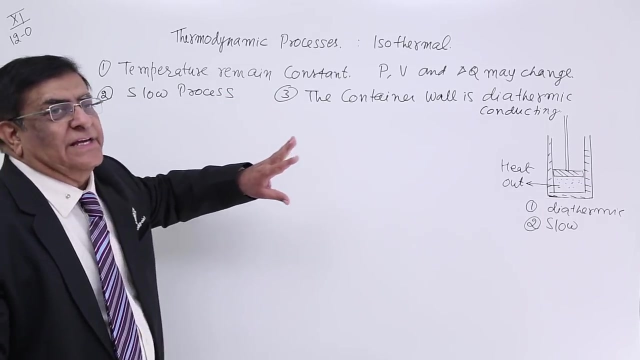 third, the container wall is diathermic. the diathermic means thermally conducting, conducting ok. these are the conditions when a process in the nature will be isothermal process. now, in this isothermal process, there are other things we can make. a co2 reveal become peradiН сюда. 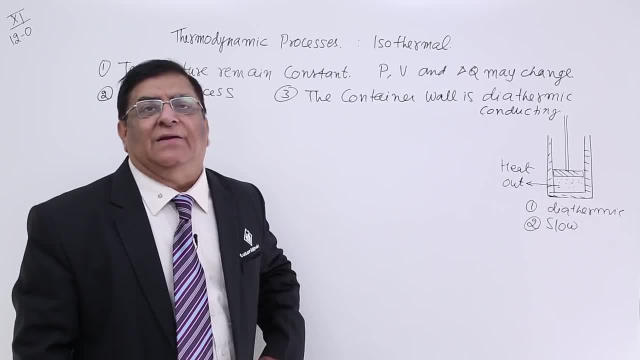 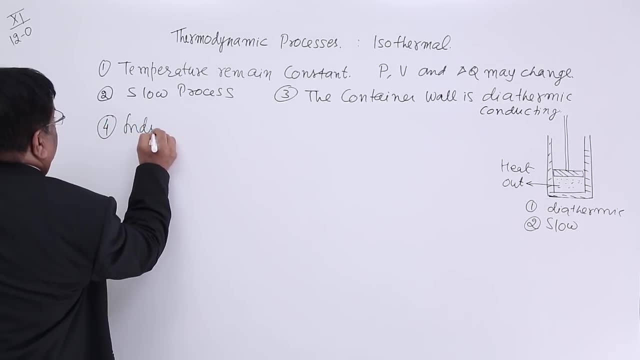 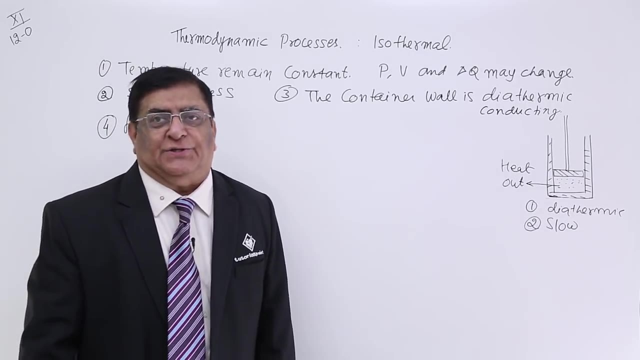 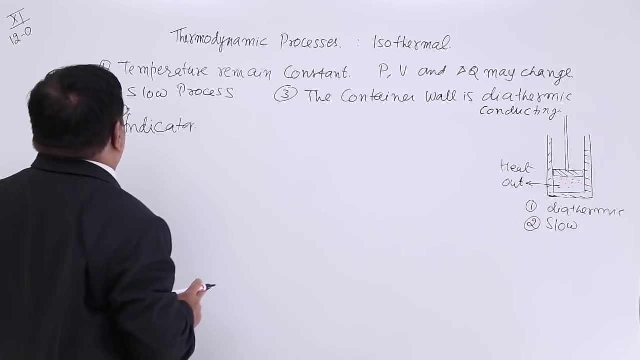 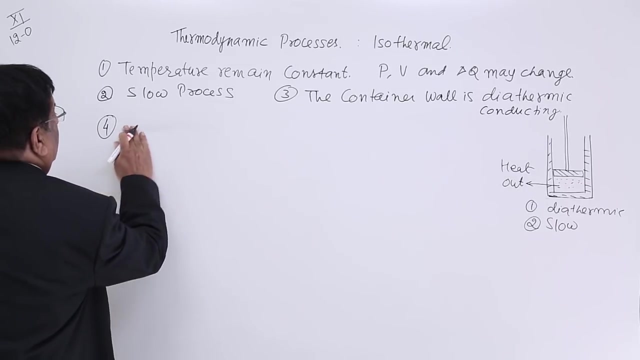 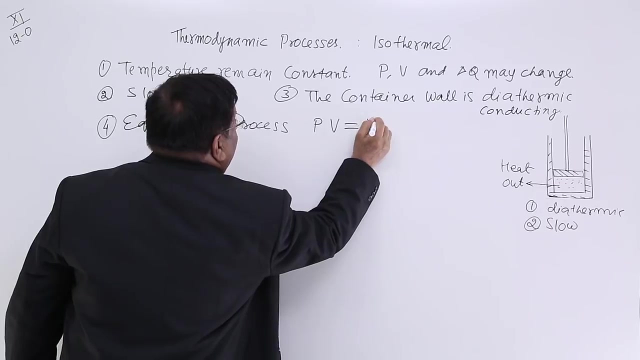 hm, hatan ada soll Greece. things we can Major V We can make an indicator diagram. Indicator means how pressure and volume are changing In this pressure and volume. see what is the equation of. first I will write equation, Equation of process. Equation of this process is: pressure multiplied by volume always remain a constant. 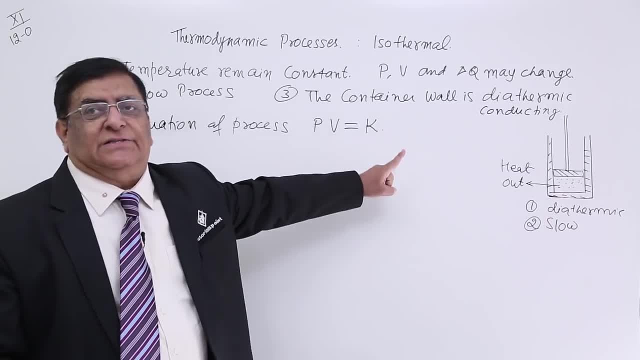 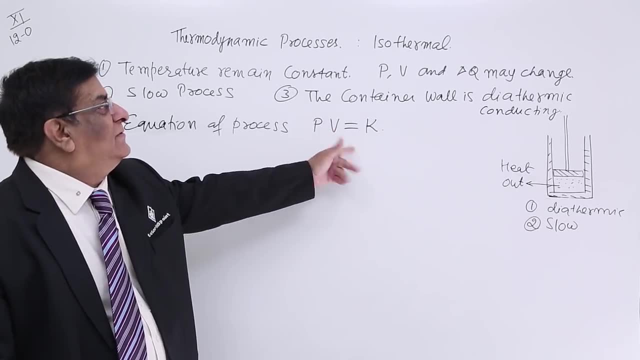 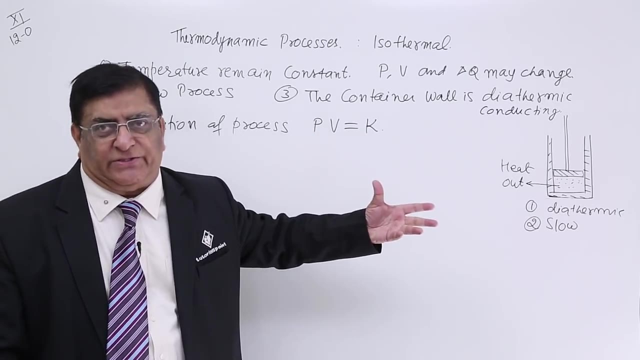 Pressure multiplied by volume remain a constant. This is process of this is equation of this process. What is not changing Temperature? When the temperature is constant, then pressure and volume remain constant. Volume have this relation. This is Boyle's law. 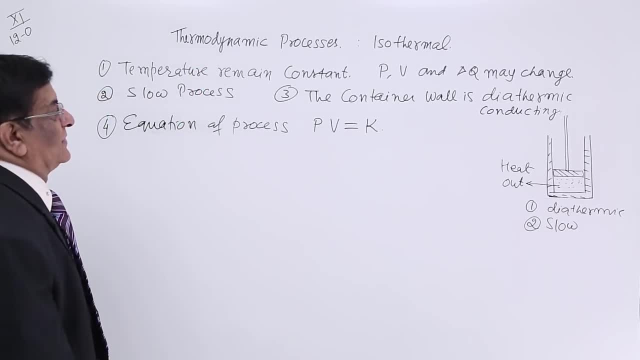 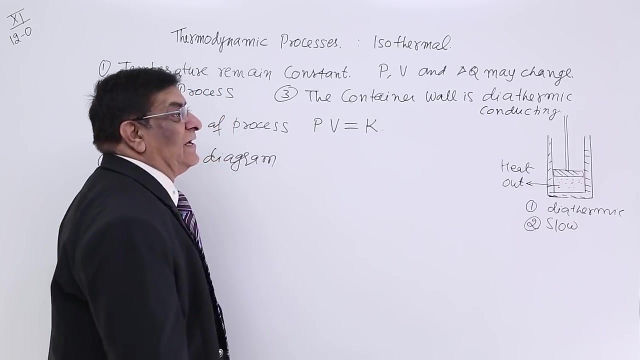 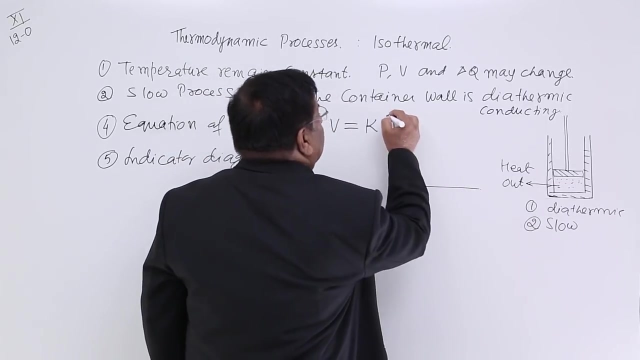 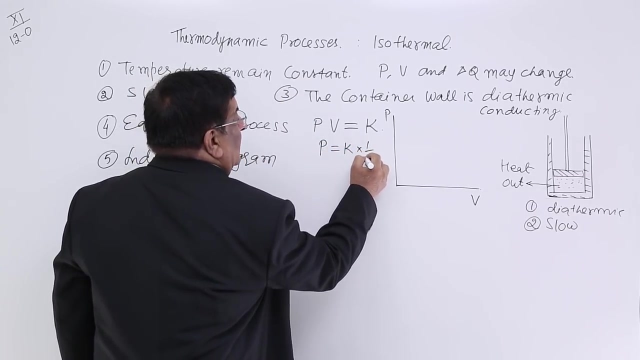 So this is equation of isothermal process. Then indicator diagram, Indicator diagram. Indicator diagram is a graph between pressure and volume. Here is the graph which has pressure and volume And here we see P is equal to K into 1 upon V. this 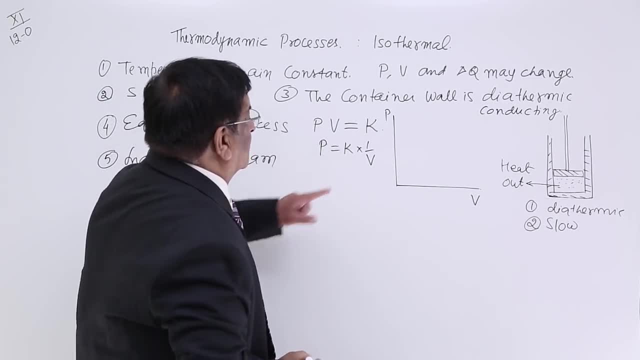 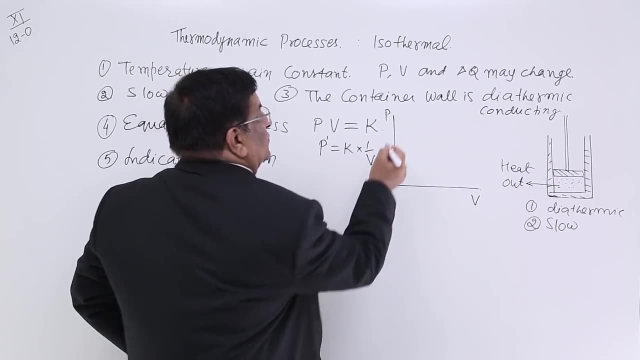 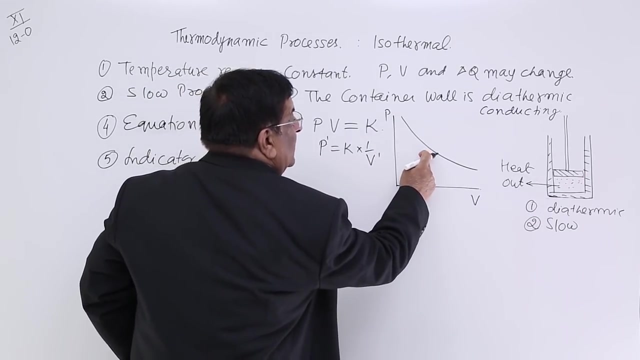 They are inversely related. So graph of such quantities when they are inversely related and power 1 to 1, then this graph comes to be inverse graph and that is like this. So this is PV graph for this, If P is this, 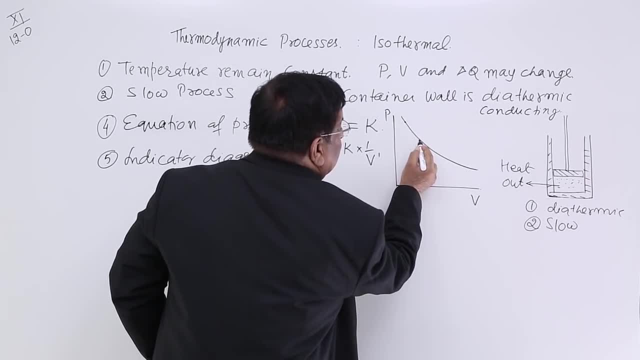 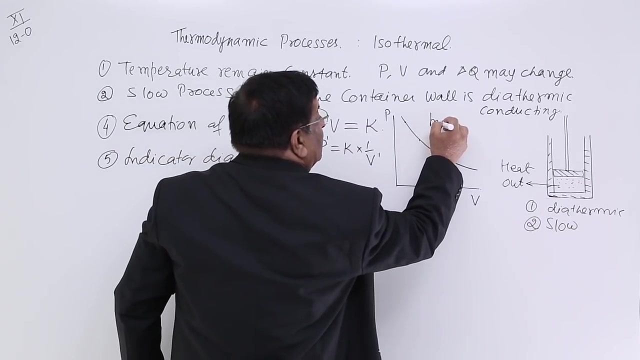 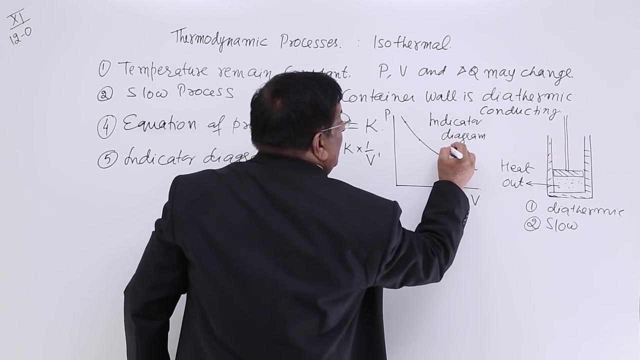 V is this much. If P is this much, then volume is this: This is P, This is P. Volume is this. So when volume is increasing, pressure is decreasing. This is indicator diagram, What we call it, please remember: indicator diagram. 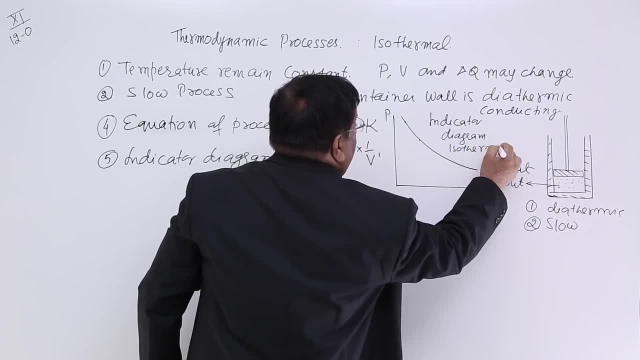 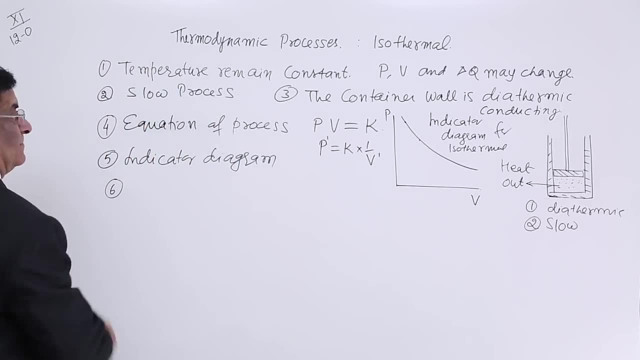 For isothermal, Isothermal, Isothermal, Isothermal, Isothermal. And you want to start this by saying that Isothermal is this much. So what? this equal to Isothermal is this much. Then you do it. You see, this is the correction here. 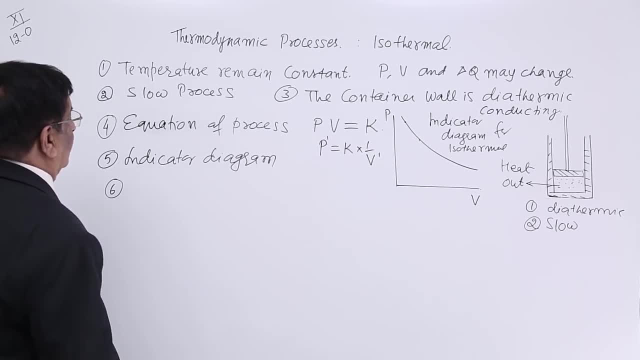 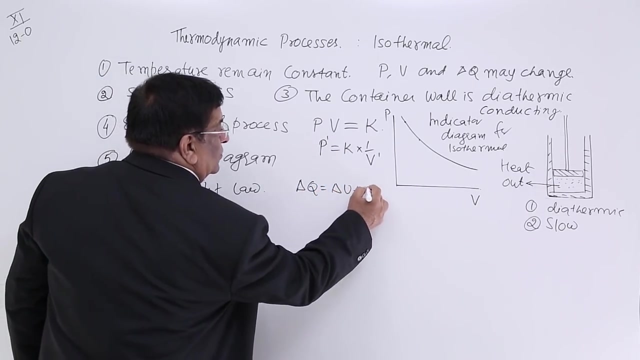 So, as you see, the lobbies are considerably higher. So this point is sort of the kisses. So let's begin here. When P equals: Oh no, you cannot Romanize it. No, you cannot. and as you go, you process theların, OMG. 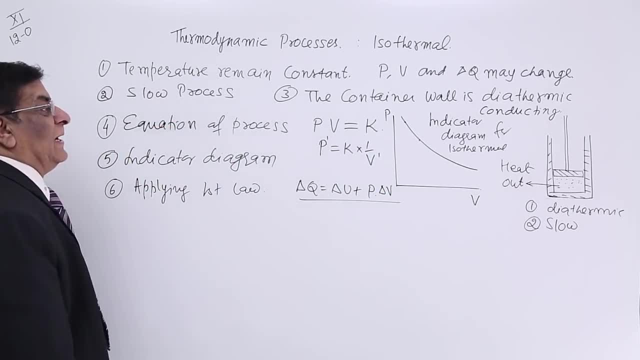 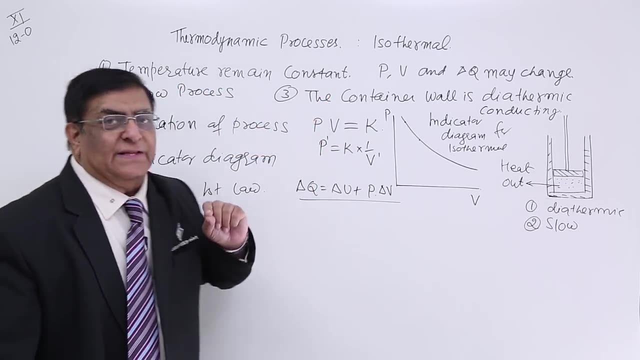 The arrow is going to be like this. It doesn't have to be like this, This way, Right? Okay, Then Here in isothermal, our condition is: the temperature remain constant, And when the temperature of a gas remain constant, what is zero? 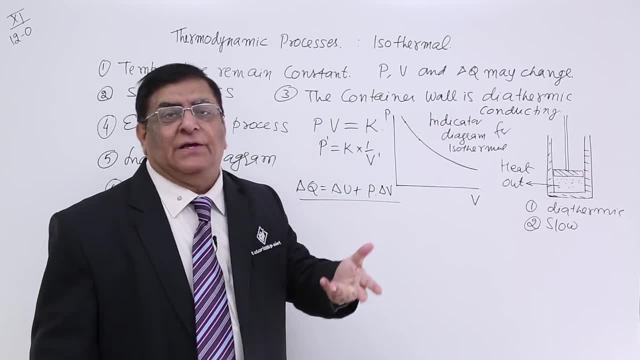 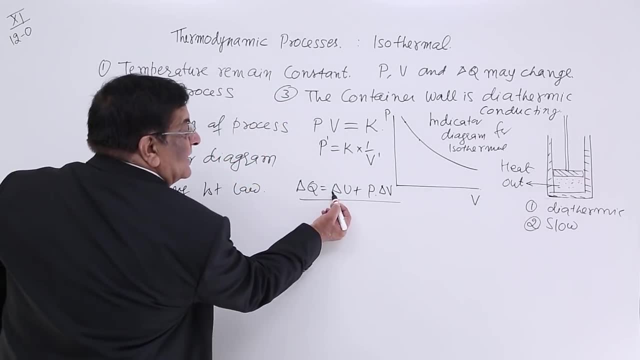 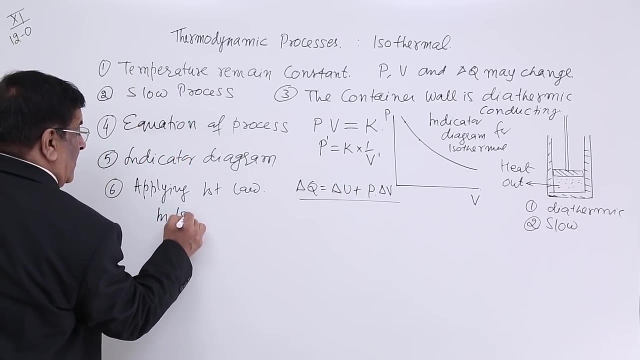 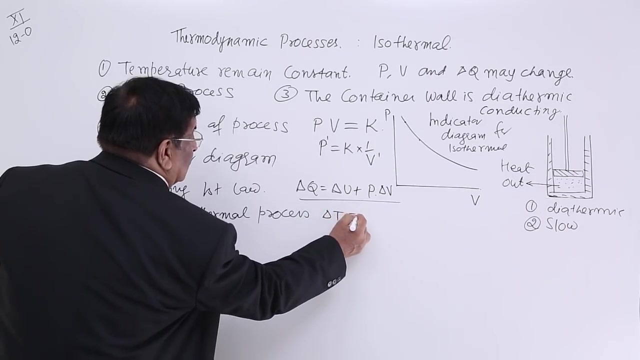 Answer: its internal energy changes are zero. If the temperature is not changing, that means internal energy is not changing. So change in internal energy, delta U is zero. So in isothermal process delta T is equal to zero. Therefore delta U is equal to zero. 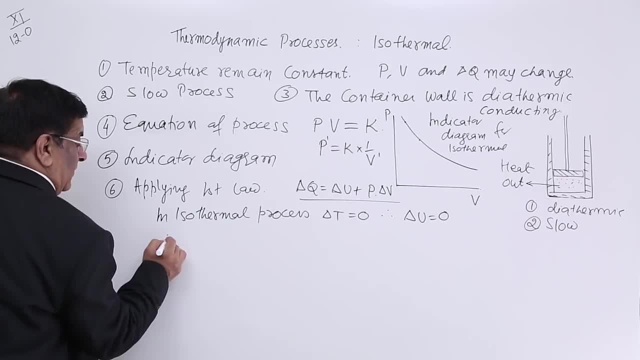 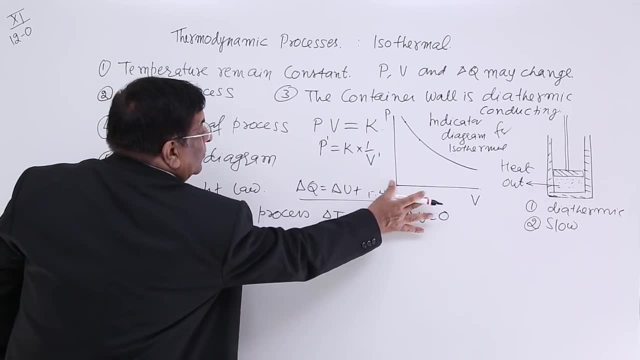 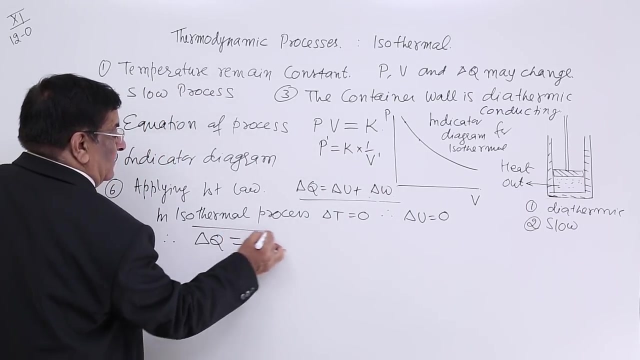 And the relation is now therefore delta Q. all the heat given is used into P, into delta V. What is P? into delta V? This is work done. So delta Q is equal to work done, And this is a very important result. 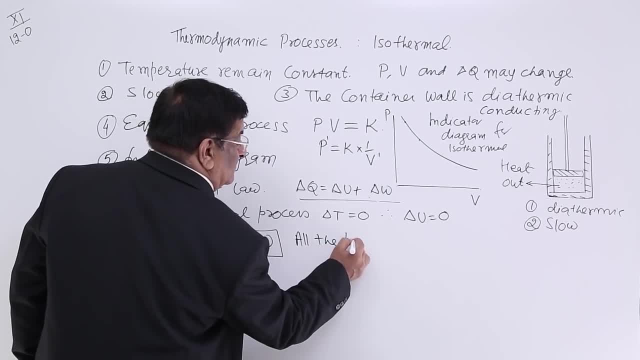 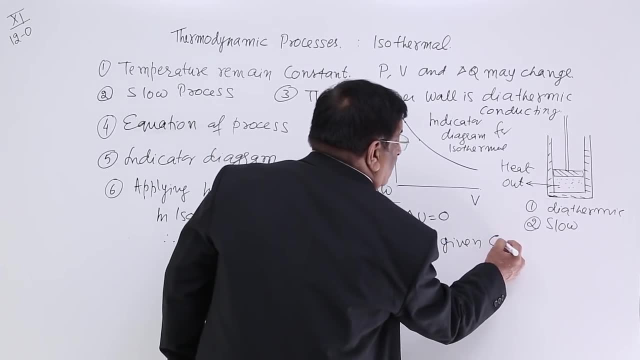 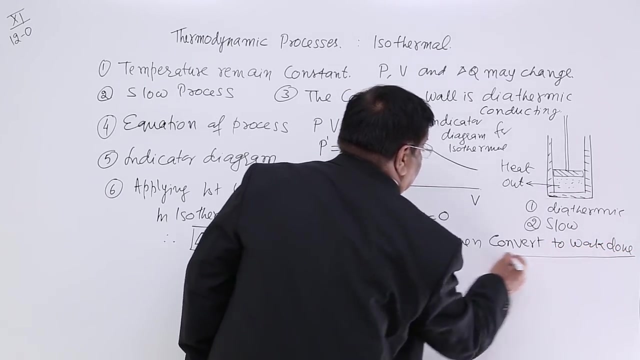 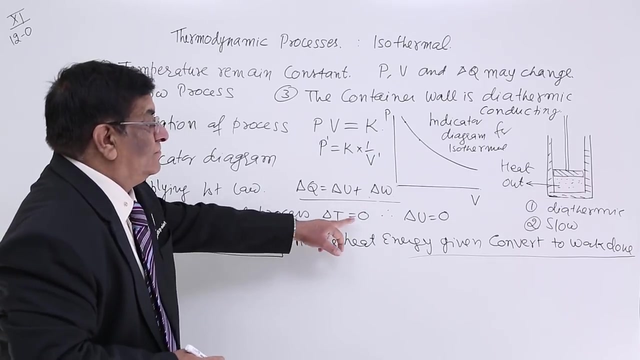 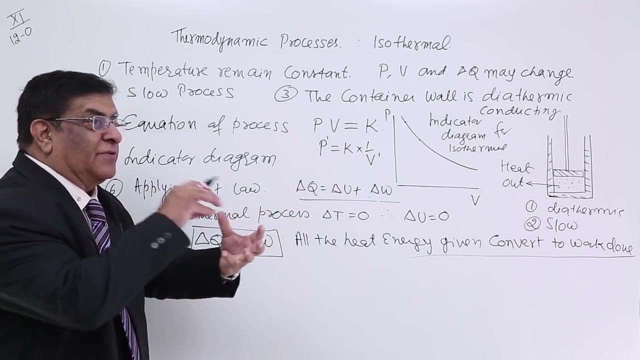 It says all the heat energy given, all the heat energy given, convert to work done. Yes, None of the energy, None of the energy is wasted in raising the temperature And for changing the internal energy. All the energy we have given from outside that is used for doing the work. 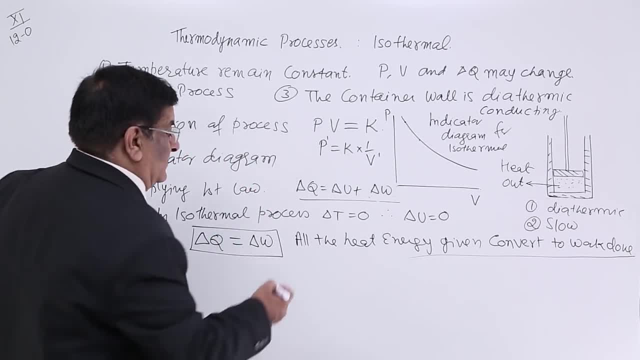 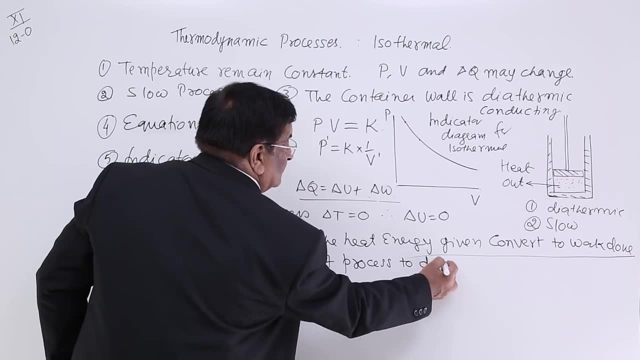 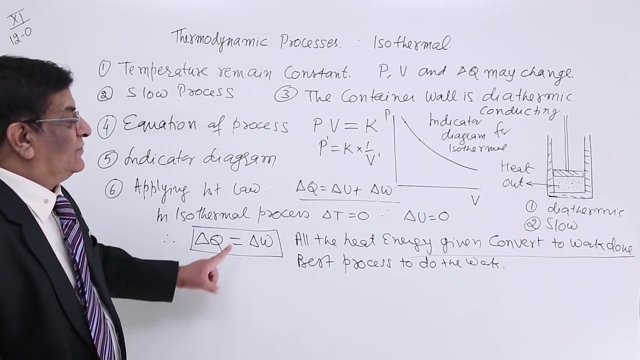 So this is the best process when we want to do the work, Best process to do the work. So the work, The work is done. in which process? The work is done in isothermal process, Because here the energy given is converted into work done. 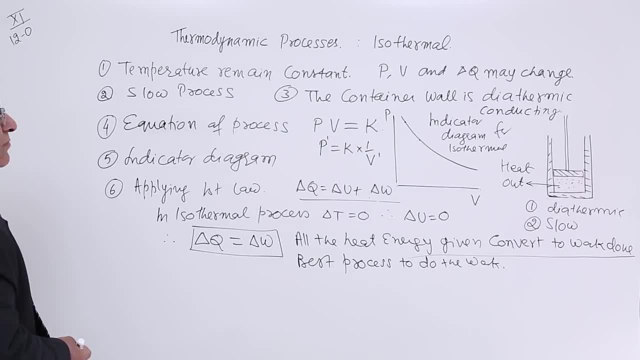 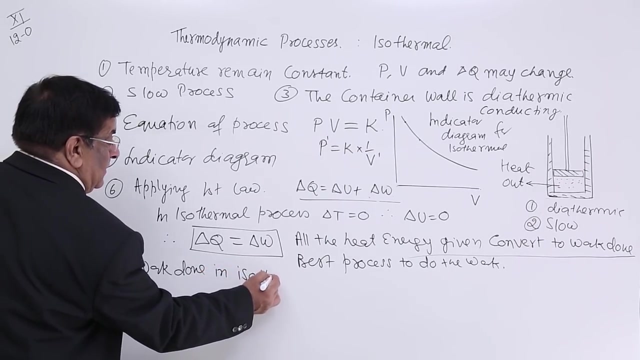 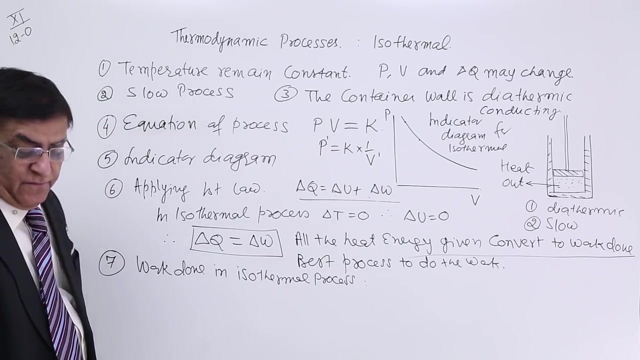 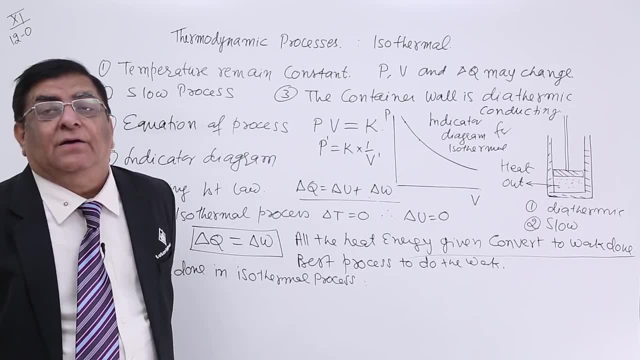 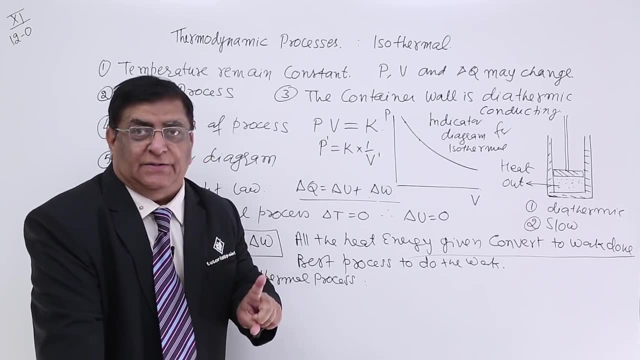 Yes, Ok, For calculation of this work done. We know that work done is calculated by force into displacement. So if you want to calculate force into displacement, we have already done that. the work done is equal to P into change in volume. 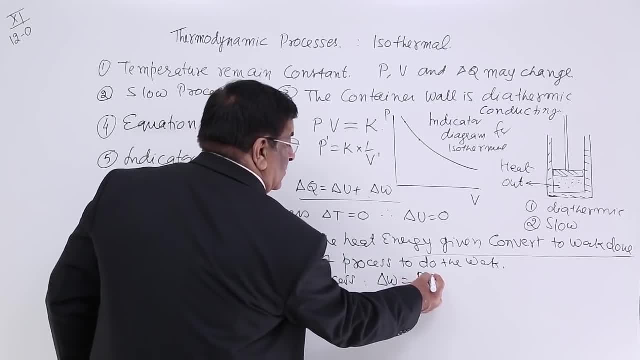 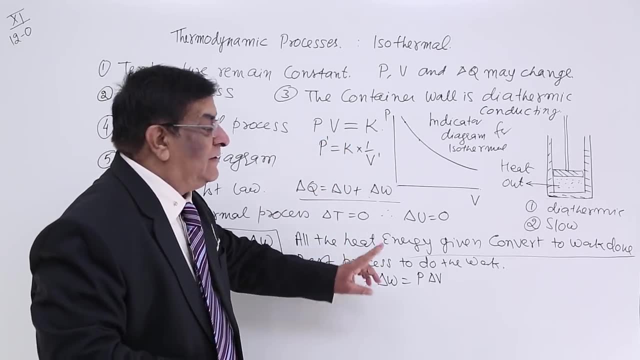 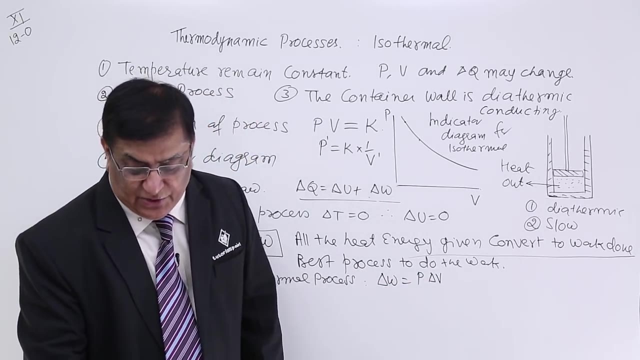 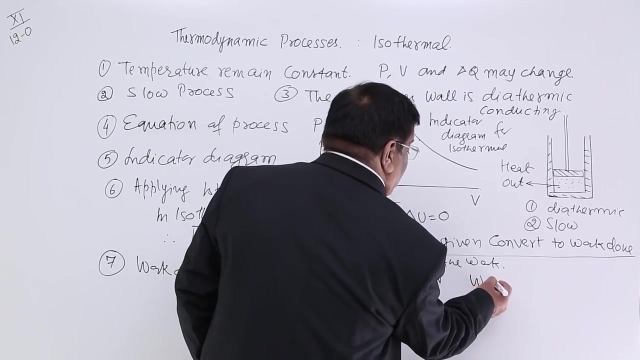 Small work done is equal to P into change in volume Because we are not raising any energy. Yes, Yes, Yes, any temperature, all the heat given is used in the work done. ok, delta w- we know it is p into delta v. so total work done is how much so total work done when we are changing volume? 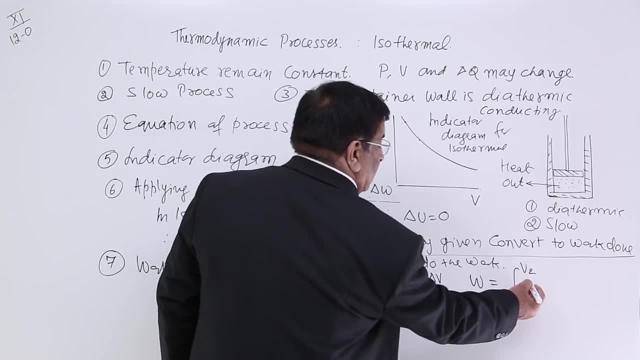 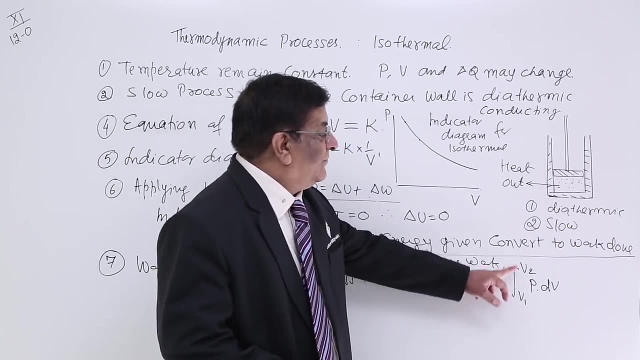 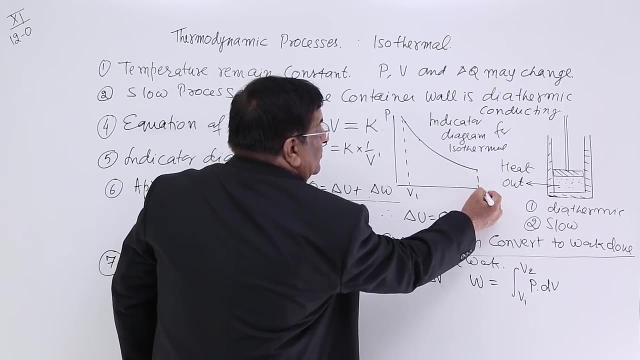 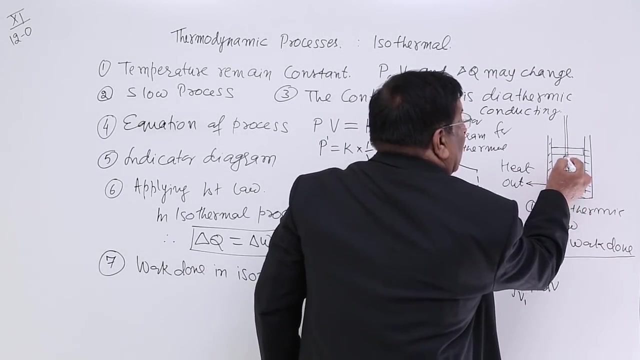 from v1 to v2, then this is integration of p into dv. this is the work done when the volume is changing from v1 to v2- initial, how much is the volume v1? final, how much is the volume v2? we have compressed it from this position to this position and some work is done. this: 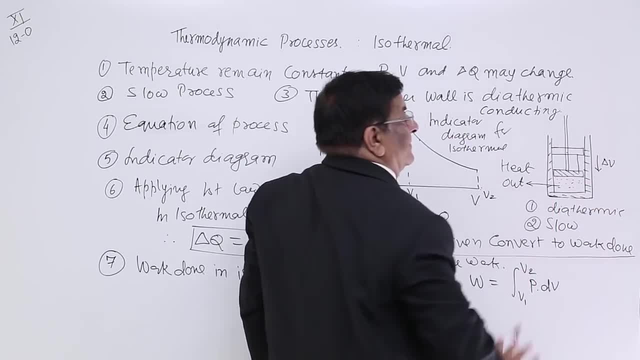 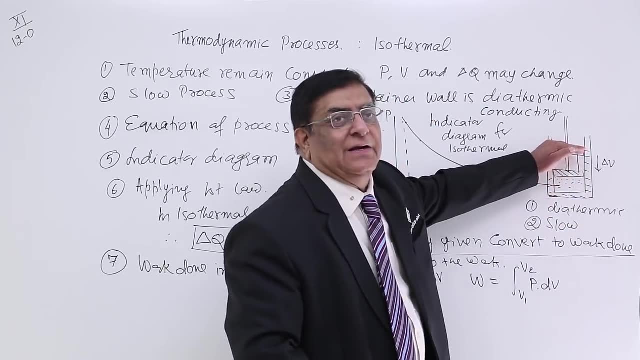 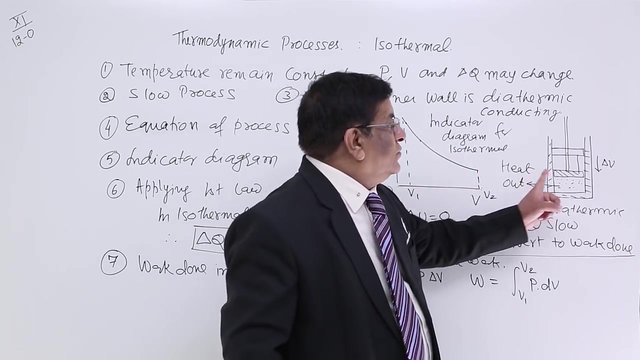 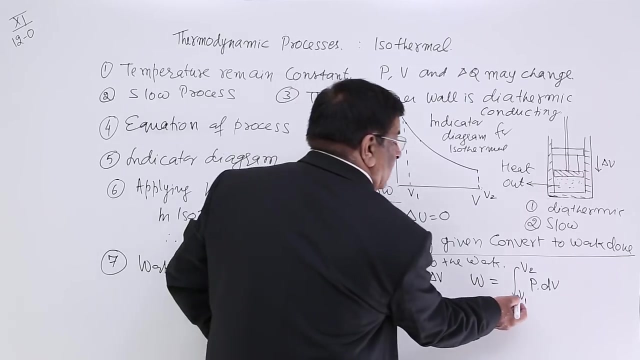 is the change in volume and some work is done this way or the other way. if we have given it heat, then it has expanded here and some work is done. ok, the temperature is not allowed to change. so because it is isothermal process, so the work done is calculated by change in volume. so work is equal to p into dv, v1 to v2 and 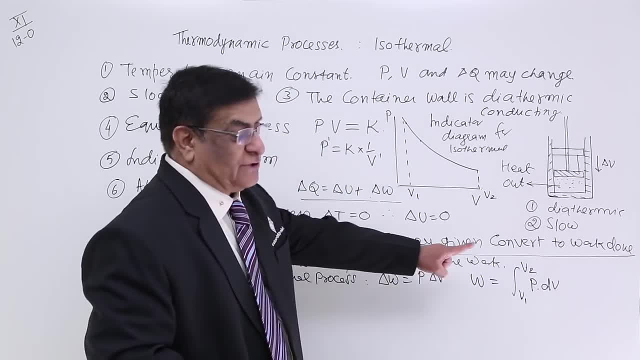 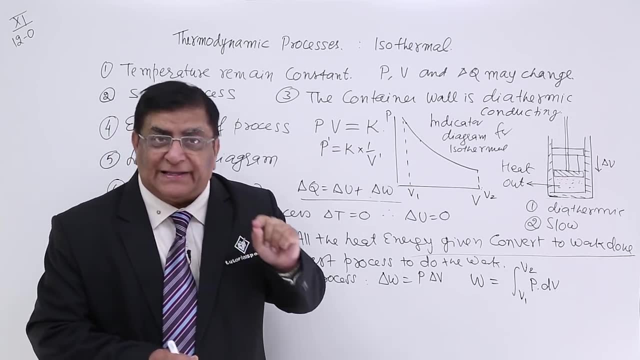 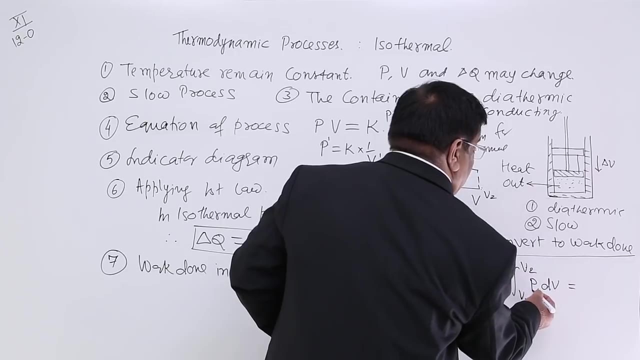 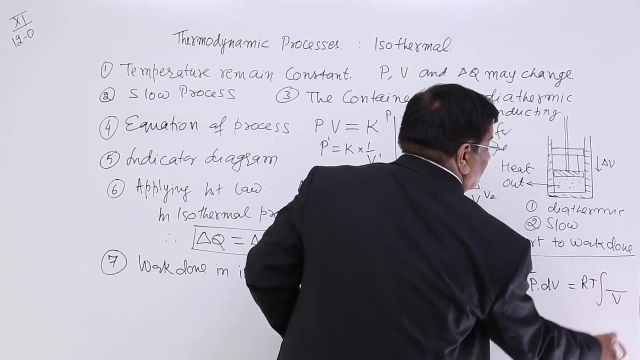 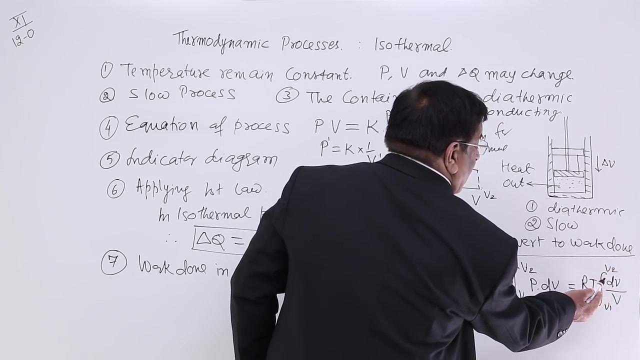 here pressure is a function of volume and that function is: pv is equal to rt. by that, pressure is equal to rt upon v. so this we can write as rt upon v. rt is a constant and v upon v remain inside, and here it is dv, v1 to v2. now this is v to the power minus 1 into dv, and we have to do the integration. 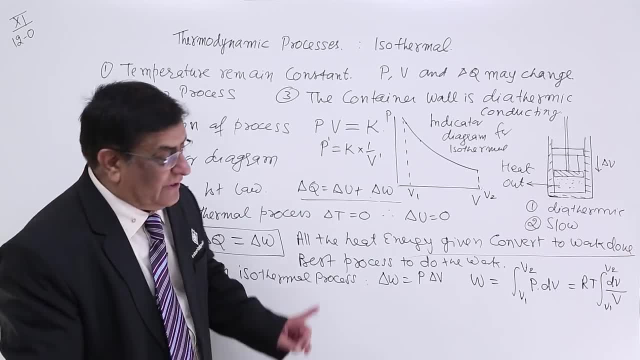 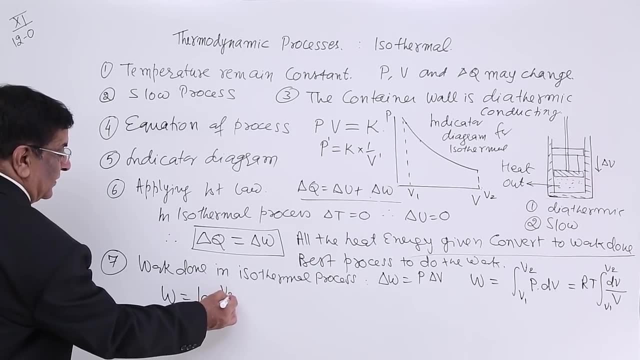 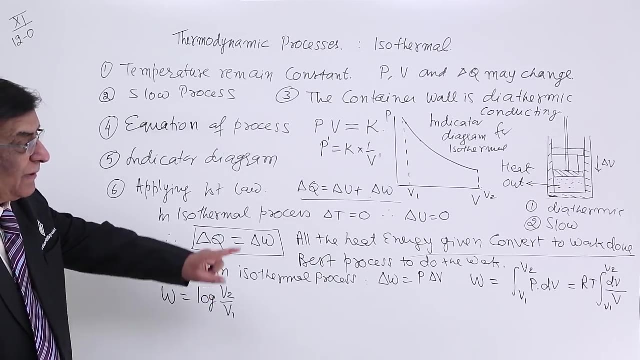 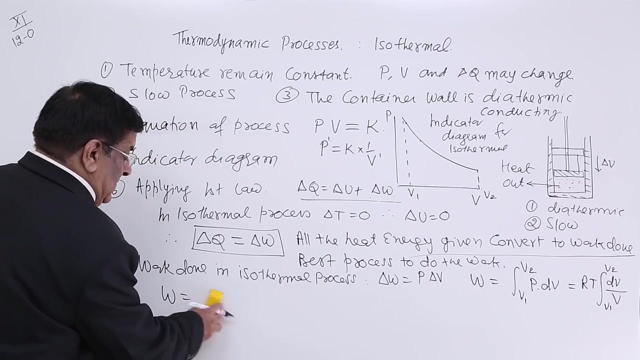 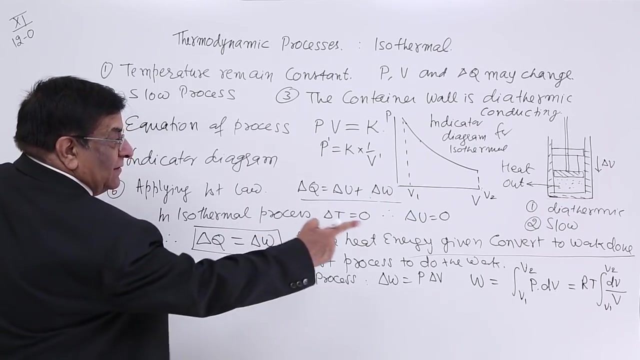 when we do this integration, what is the term we get? we get log. so total work done is equal, equal to log, V2 upon V1.. This is what we get from here, multiplied by RT. So multiplied by RT. I will write that first. So this is equal to RT and V 1 upon V. integration will. 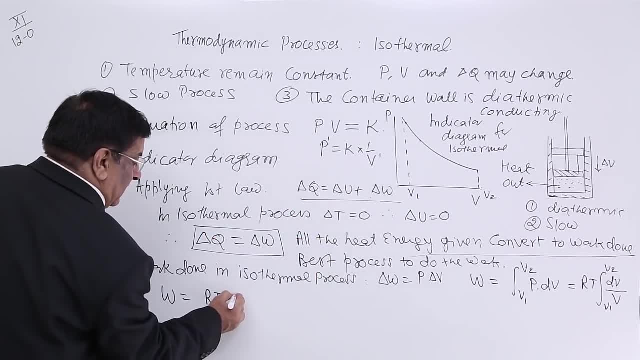 be log V and we put the limits. So this will be log V2 minus log V1 and that is equal to log V2 upon V1.. These are 3 steps together. This is for 1 mole of gas. If the gas is not, 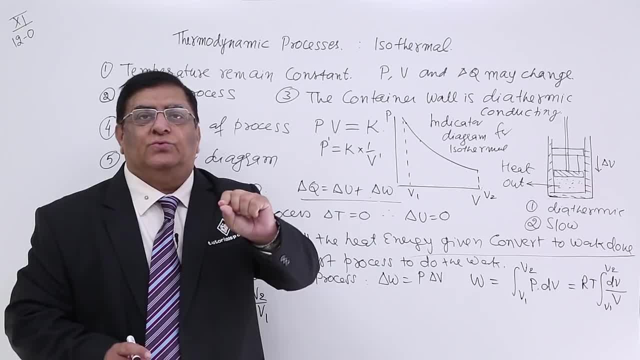 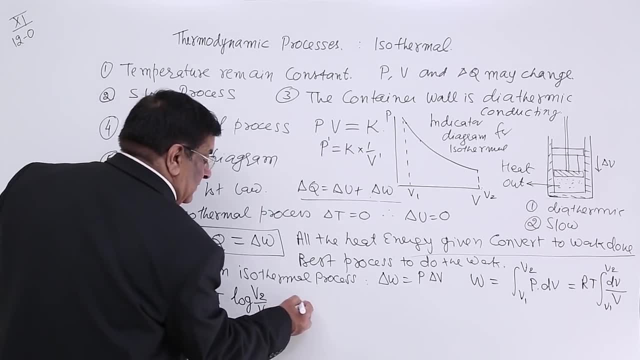 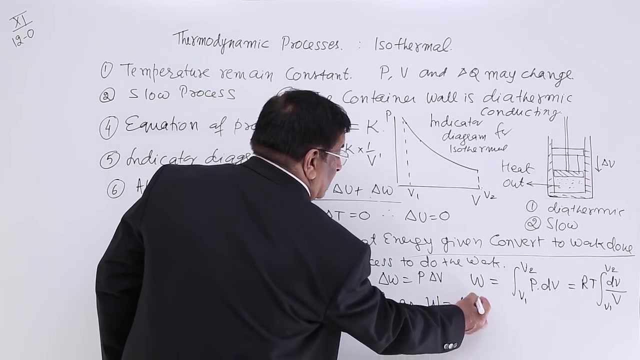 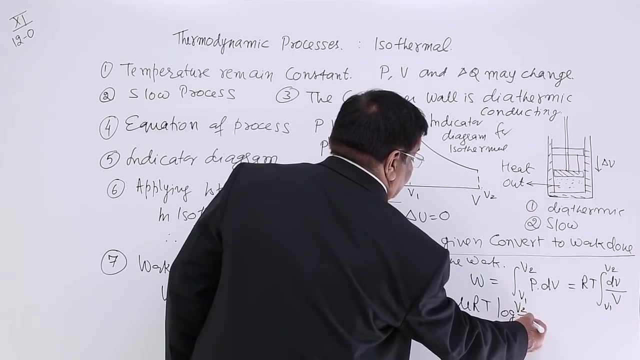 1 mole and it has mu as mu moles of gas. then we can again change it and we put that mu here right here for For mu mole of gas, the work done is mu RT log V2 by V1.. This is work done during isothermal. 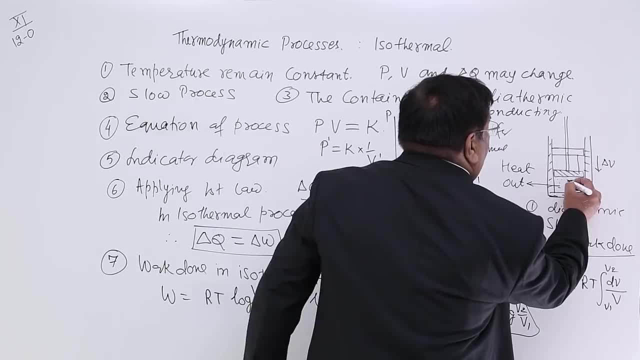 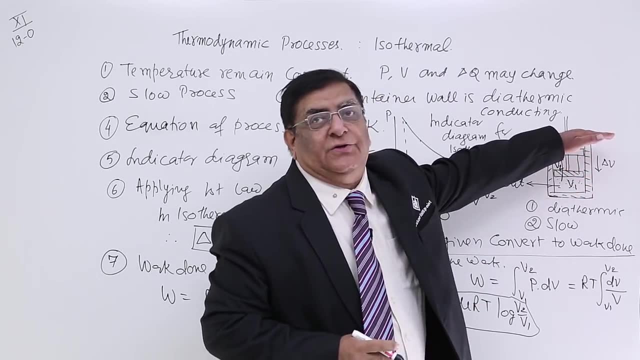 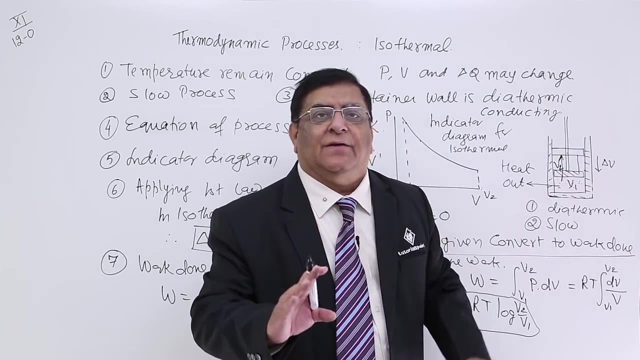 process The volume has been changed from V1 to V2.. When the volume is changed from V1 to V2, either by giving the heat or by putting mechanical force, by anything keeping temperature constant, then how much is the work done in isothermal? 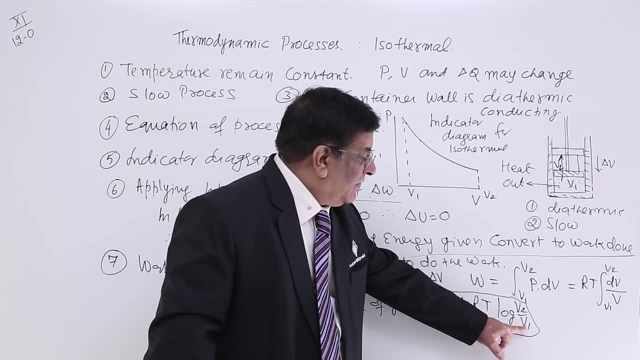 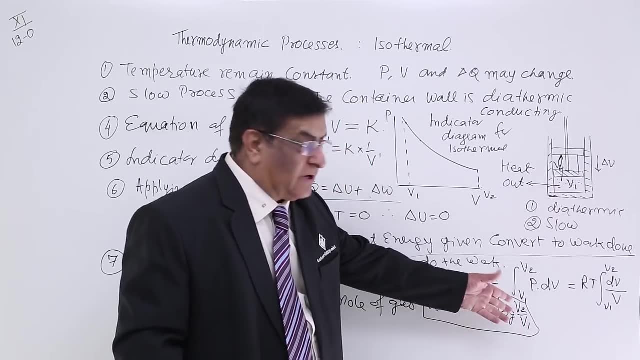 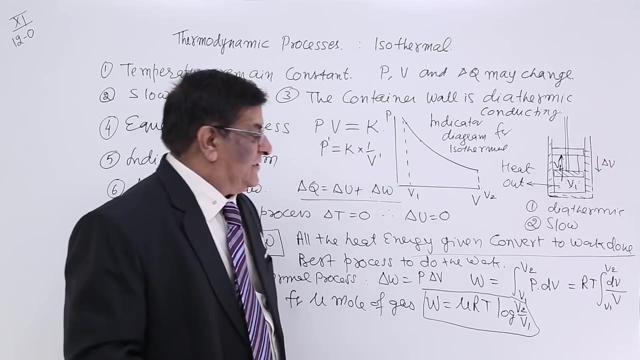 process. This is the work done. The volume changes from V1 to V2, then log V2 upon V1.. Higher is the V2, more is V2, more is the work done. It is visible here And at whatever temperature we are operating, that temperature is here. So this gives us. 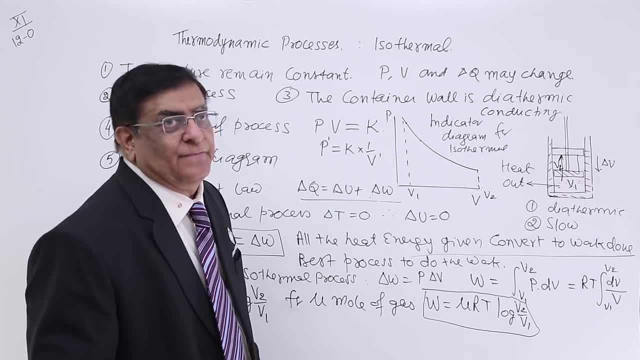 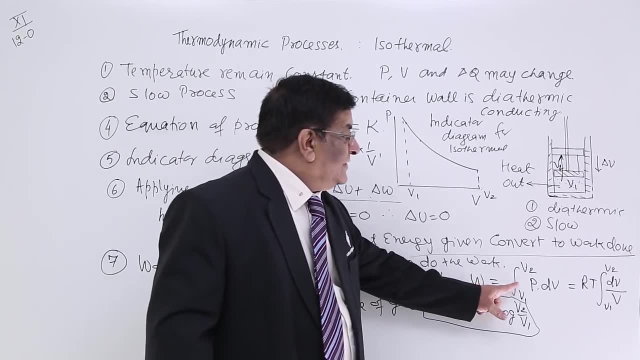 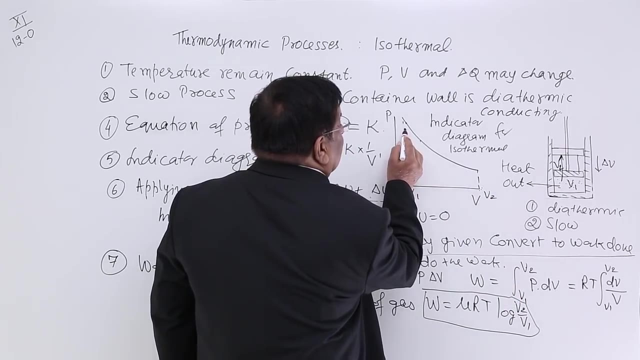 the work done by calculation. The work done can also be calculated graphically, because this is what? integration of P into d, V, from V1 to V2.. Here is V1 into V2.. And if we take this area, what is this? P multiplied by dV? So this gives us Suffice, the area. let say: 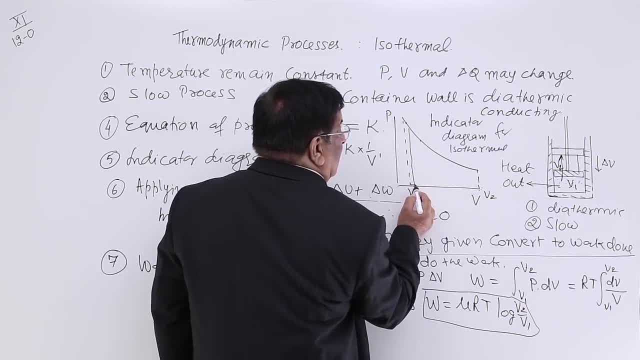 multiplied by dV. Why? Because this is called. we have calibrated sectional 거야蒸 toteed dv. Again, this is P multiplied with dv- this area, P multiplied by dv- this area. In this way, if we have this total area calculated, then this area mathematically is what P dv. 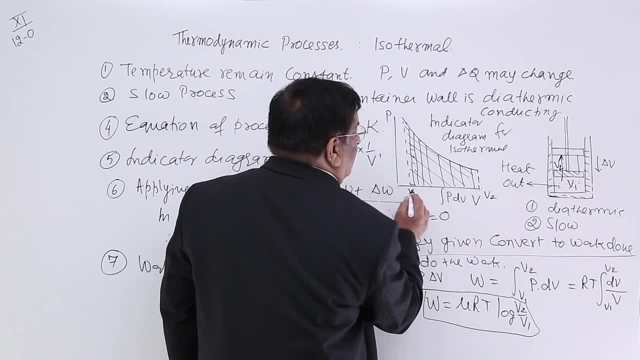 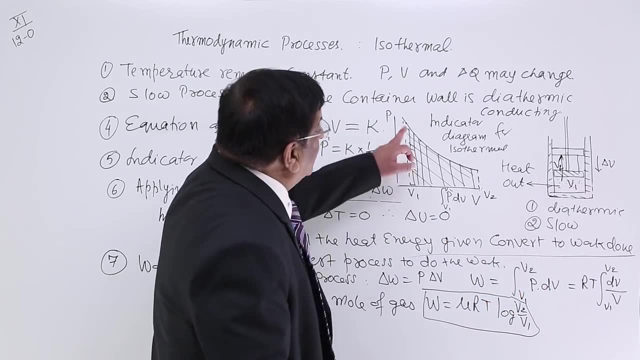 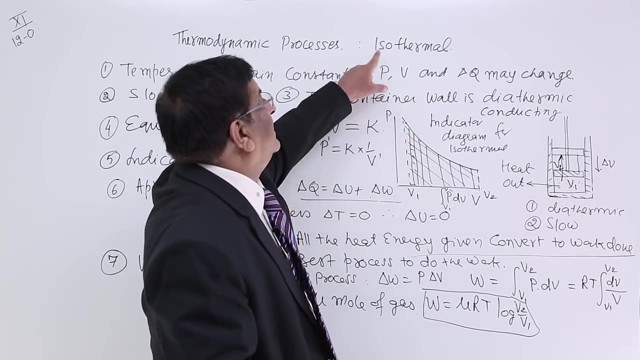 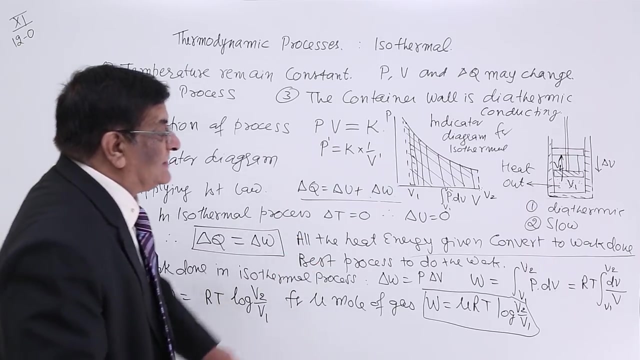 P dv, P dv, integration of that from V12, V2, V12, V2.. This And what is this Work done? So area under indicator diagram gives work done by the isothermal process. So work done in isothermal process is this mathematical expression And this is also equal to area. 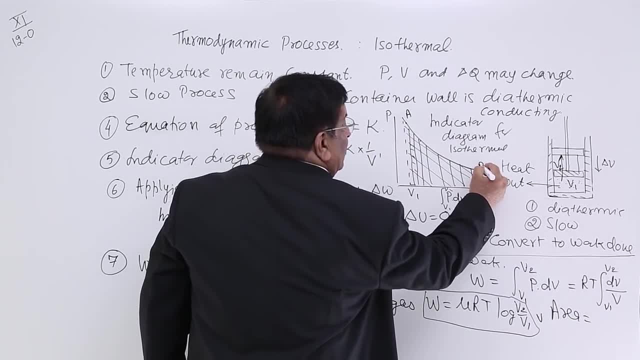 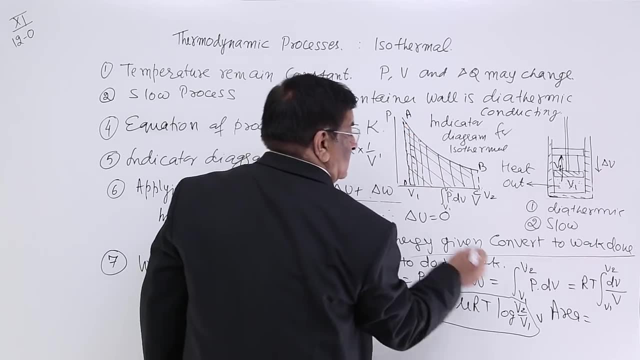 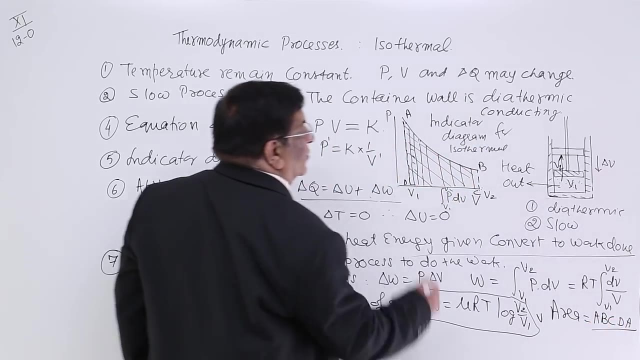 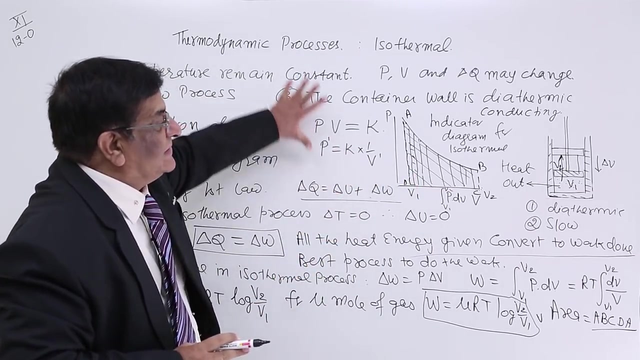 area and we can write here A, B, C, D. This point is D, So this is area A, B, C, D, A. This closed area gives the work done by isothermal process. So these are all the details of isothermal. 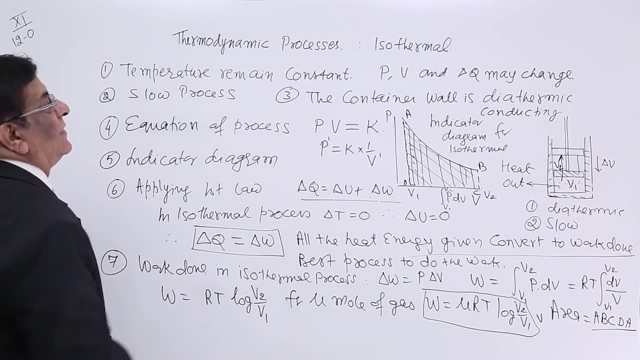 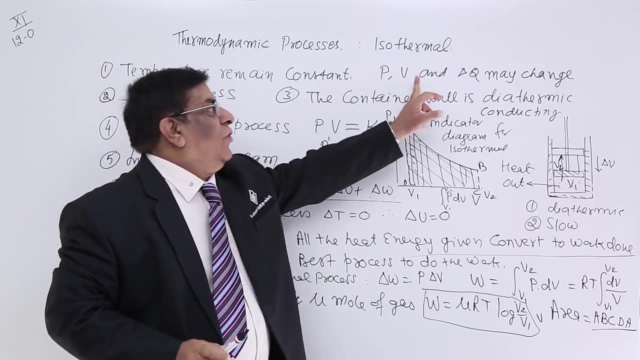 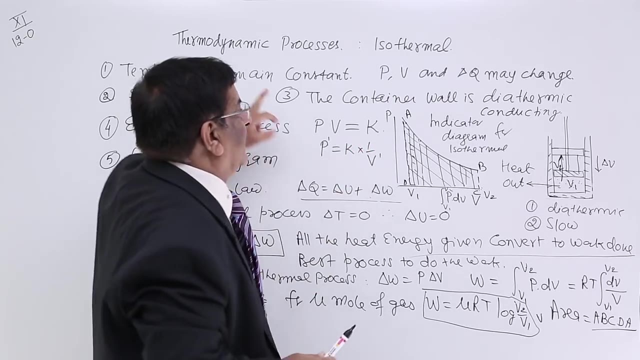 process. Once again. I repeat you in brief: Any process in the nature where temperature is not changing, pressure volume and heat given to the system may change That process we will call isothermal process. This process has to be slow process so that heat generated. 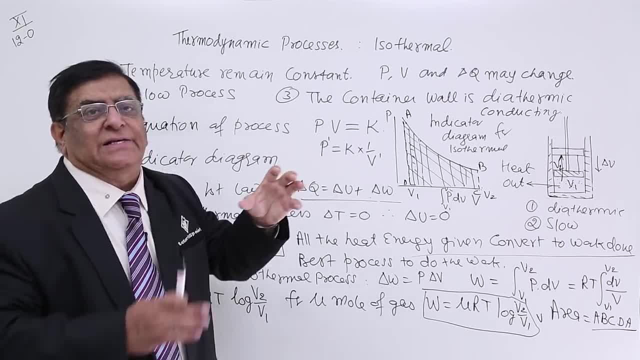 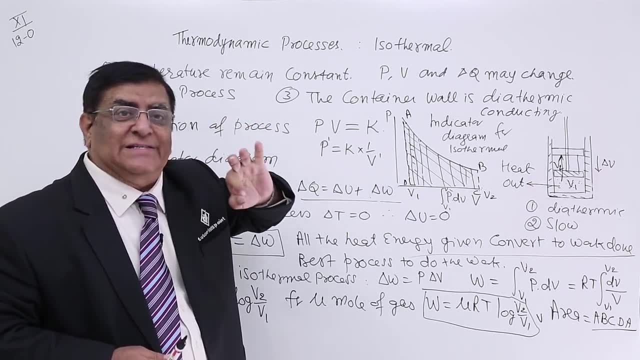 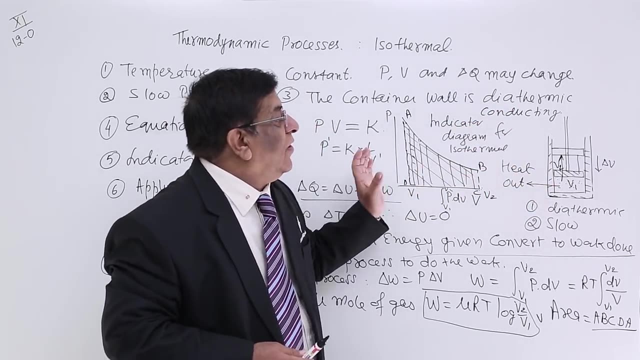 during the process or heat lost during the process is compensated by the surrounding process. It is not that heat is not generated. Heat is generated, temperature rise- But due to diathermic wall, the heat goes out or it is imported in So that temperature do not change. 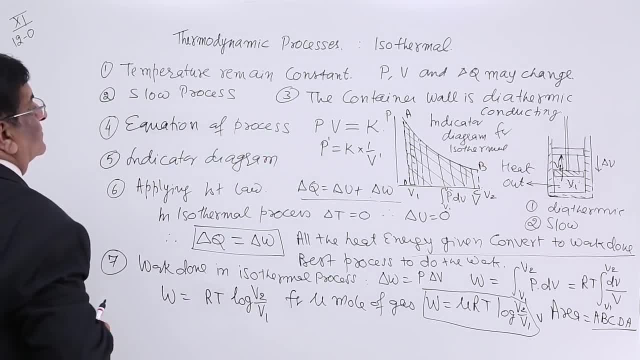 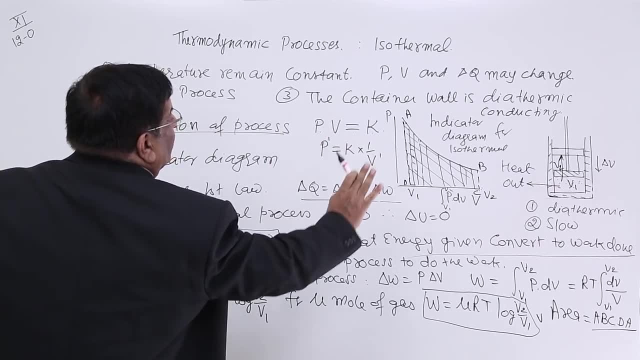 So the wall has to be diathermic. Then what is the equation of this process? PV is equal to K because P and B are changing. There is no mention of T. T is constant. Now, what is the equation of this process? PV is equal to K because P and B are changing. There is no mention of T. T is constant. Now, what is the equation of this process? PV is equal to K because Sy is equal toK. This is the equation of this process. PV is equal to K because Sy is equal toV is equal toI. I am going to dominate the information. 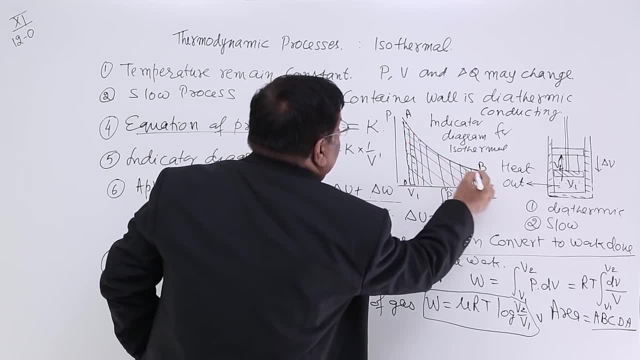 This is the equation of the first equation for 13A by 14B. What is the predominant method? What is the dominant method? Well, let us give an example of the dominant method. It is called the S celebrate voltage. well, Let us give a solution as means of 0.. 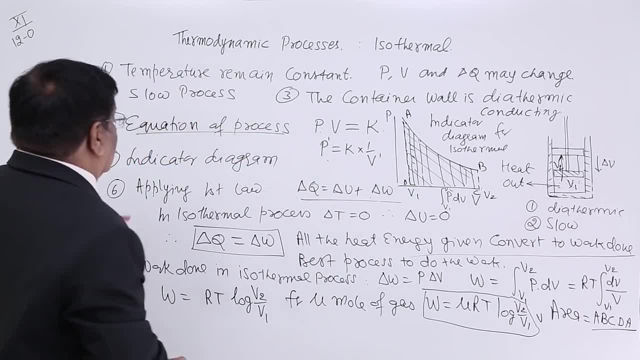 Where is this? second example? S is such that H, m, S is a P m of 1 or N, And we can這樣子 after this: all those values we have become From PL as to L times 1.. 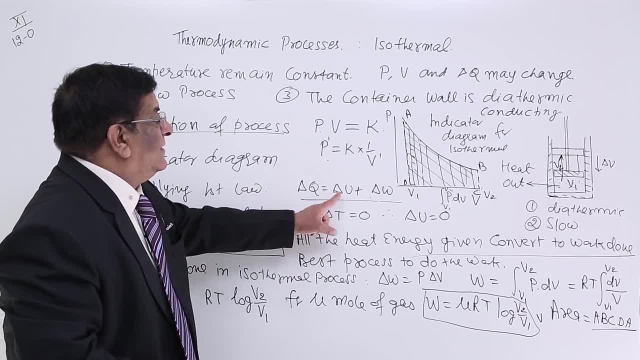 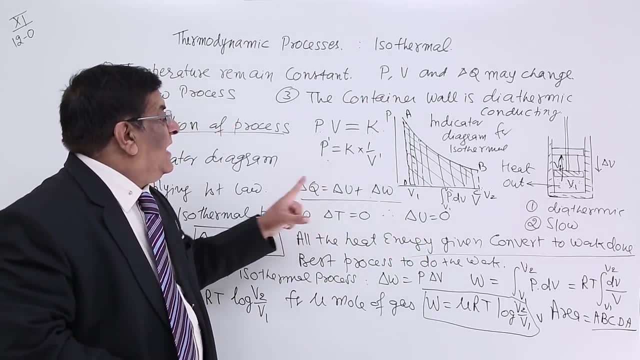 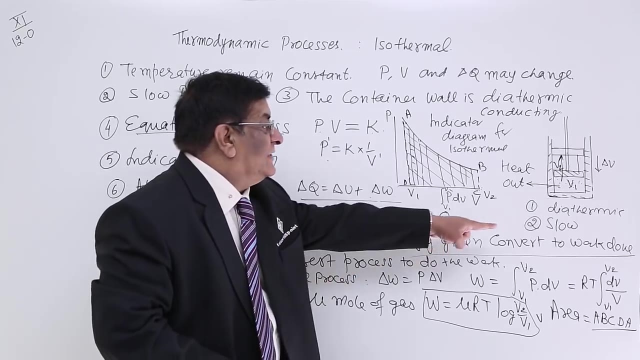 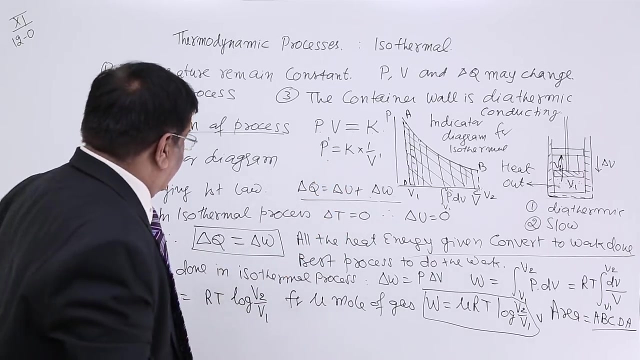 Alright, Then you know what happened after FIRST Entrance. t, which means 15,, K and C. heat energy convert to work done, and this is the best process to do the work. Only in isothermal process work is done. Now work done in isothermal process can be calculated. 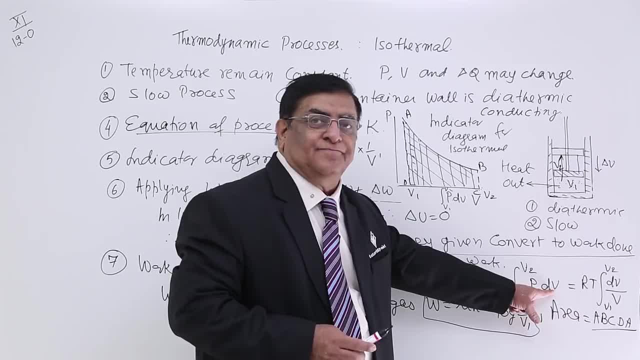 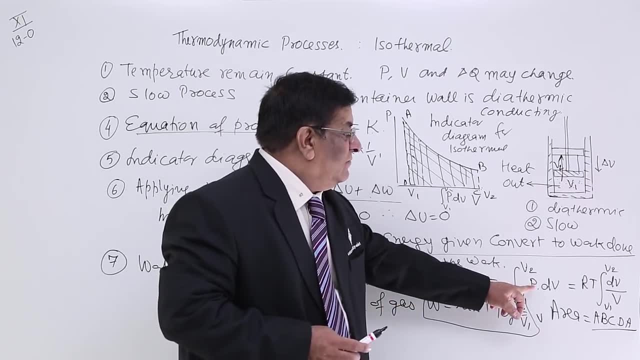 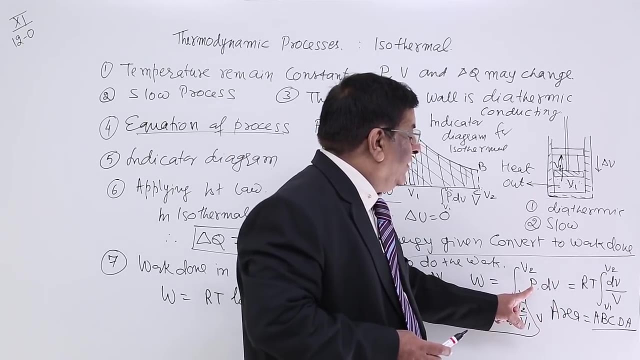 as integration of P into dV, That is, change in volume multiplied by P, gives us the small work done and integration will give the total work done from V1 to V2.. And PdV, P is from. PV is equal to RT, P is equal to RT upon V And when we integrate this we get log V and